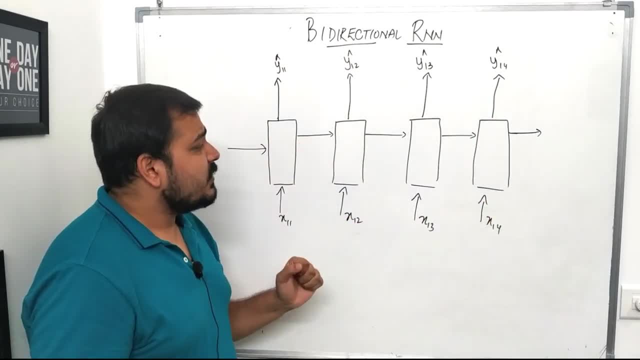 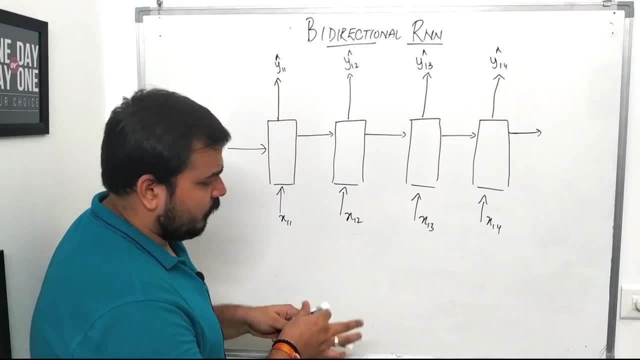 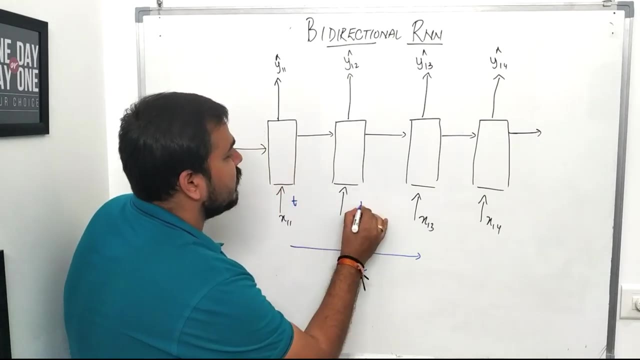 a simple RNN architecture. Now, considering this particular RNN, you can see that, guys, we are passing input words X1, X2, X1-2, X1-3 and X1-4.. Remember, this is basically my time axis. So this is basically at time t, this is at time t plus 1, time t plus 2 and 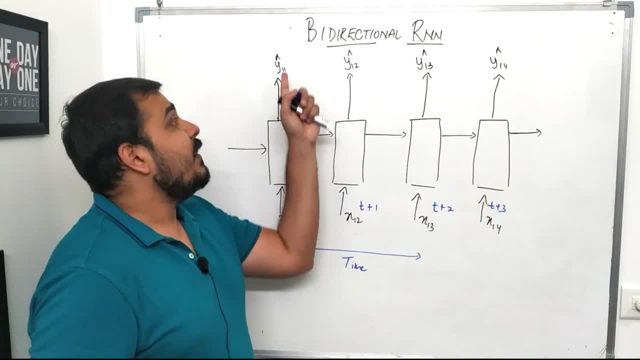 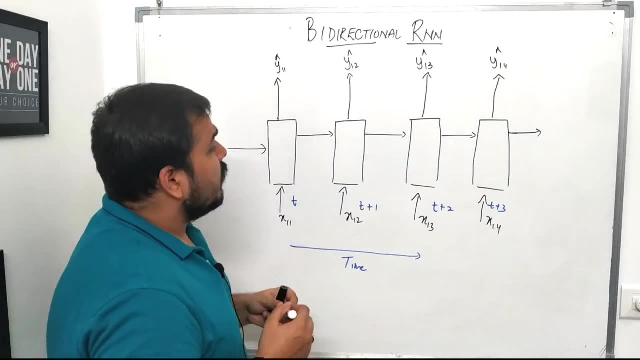 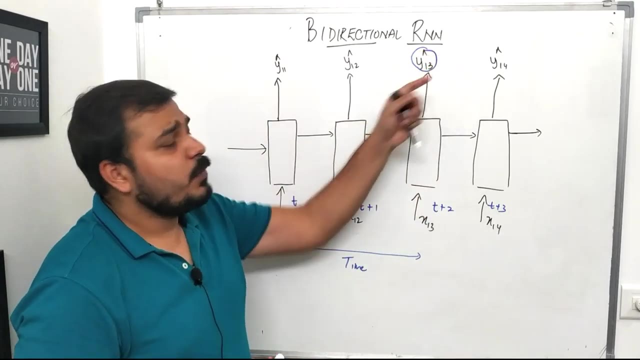 time t plus 3.. And considering this, we also have an output: Y11 hat, Y12 hat, Y13 hat and Y14 hat. Now, if we consider, let us consider this particular output, guys, Now remember, this particular output is right now dependent. if I just consider that, in order to come to 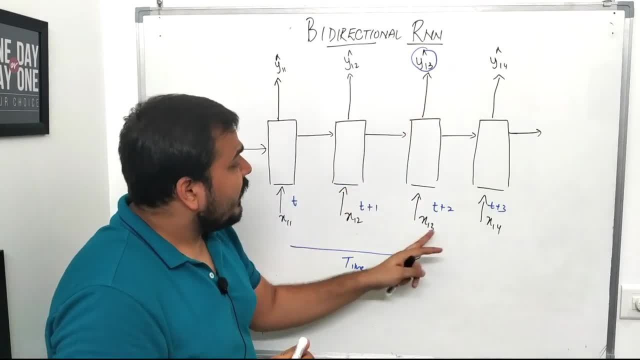 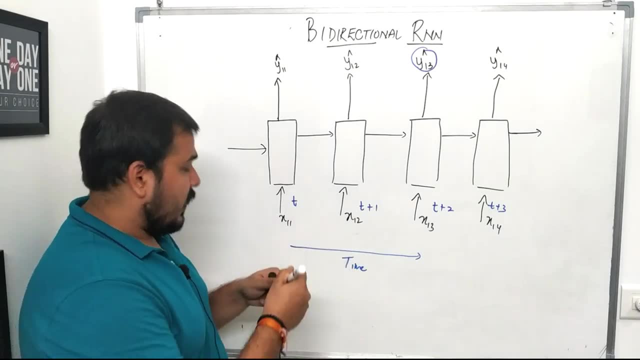 compute the output of Y13 hat. we need to have the information of X13,. we need to have the information of X12, we need to have the information of X11. And this is basically X0. guys, Now, obviously this information is getting passed. right, it is getting passed. 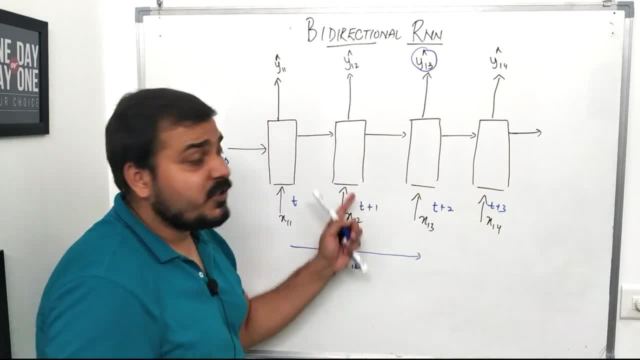 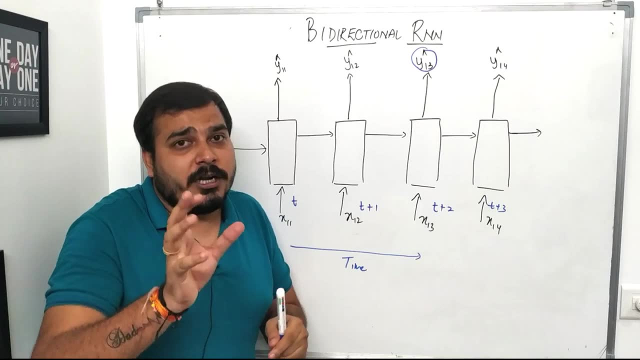 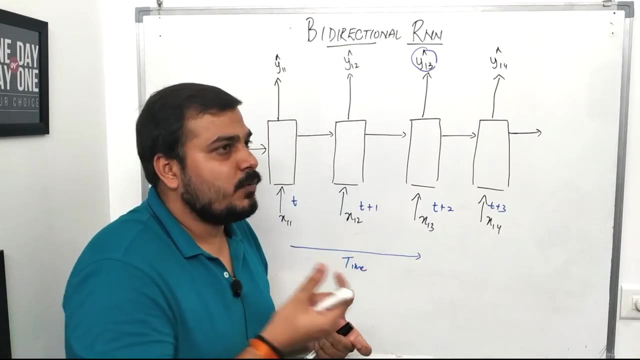 along with the output. this is also getting passed. You can see X12 information is also getting passed. X13 information is also getting passed. So finally we will be able to compute Y13 hat. But what if This particular output is dependent? the future words: okay, so it may. if I take as an example, suppose he likes eating. I want to find. 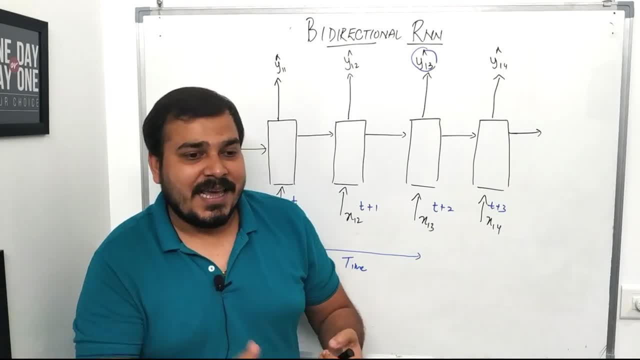 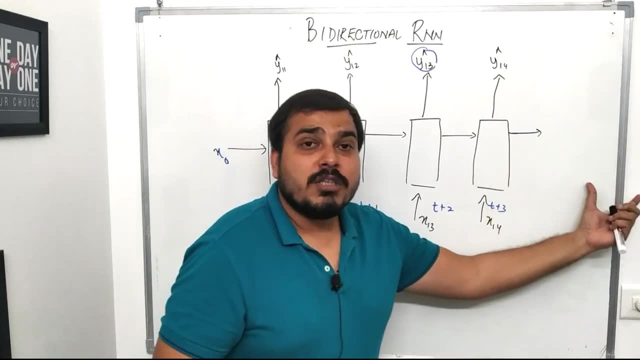 out the next word. now there may be various words. he likes eating apple, he likes eating banana, he likes eating chocolate. it can be many words. so based on the future context, whenever there is a dependency to compute the output after this word, you know it may be dependent on the future word. 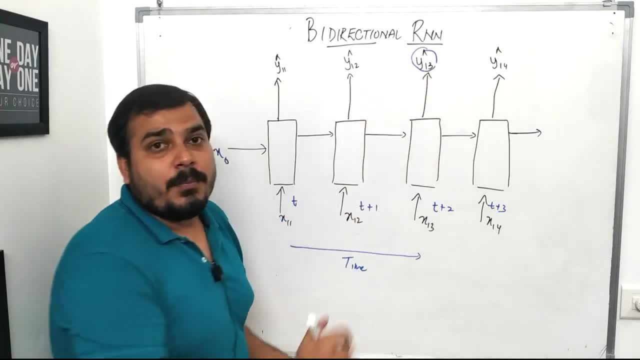 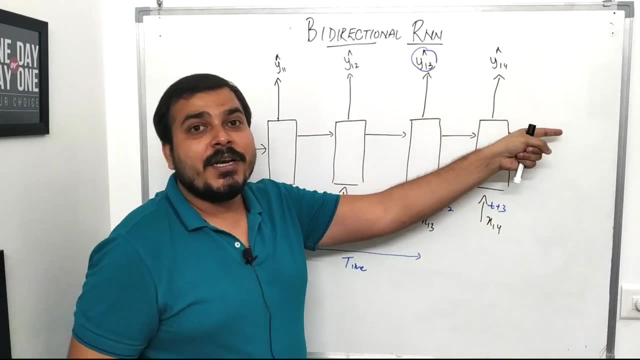 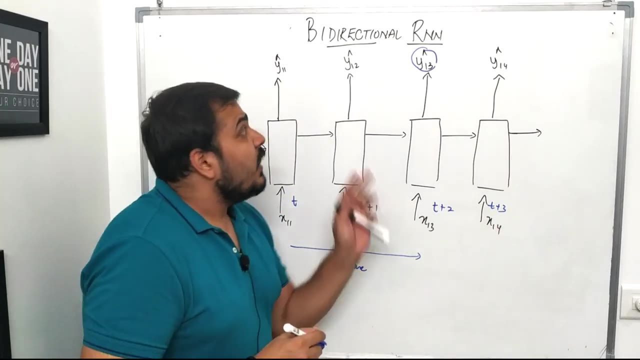 itself. so, considering this in order to solve this particular problem, because right now I'm just getting and remember this RNN, all the information are passing unidirectional way. okay, we cannot get the information of the future words right. so, considering this, we have a concept of bi-directional. 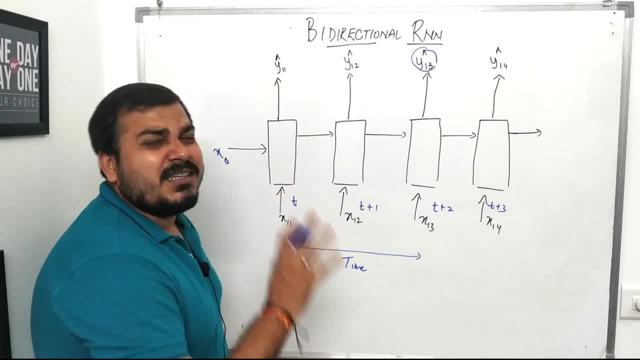 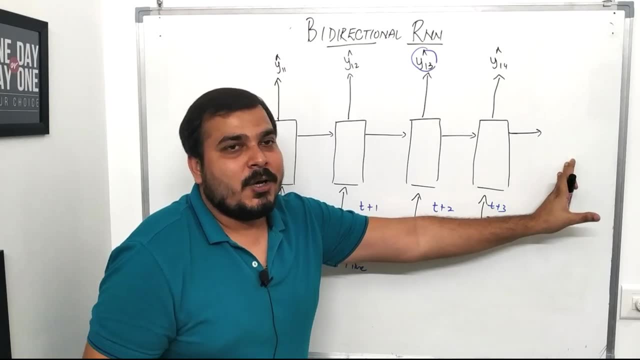 RNN. now, what is happening in bi-directional RNN? nothing, guys. it is pretty much simple. the same RNN. we will try to take it, okay, I'll say it as backward layer RNN. okay, so this is the same RNN. we will try to take it. okay, I'll say it as backward layer RNN. 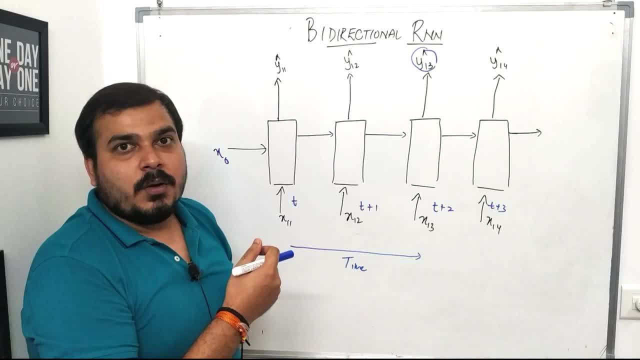 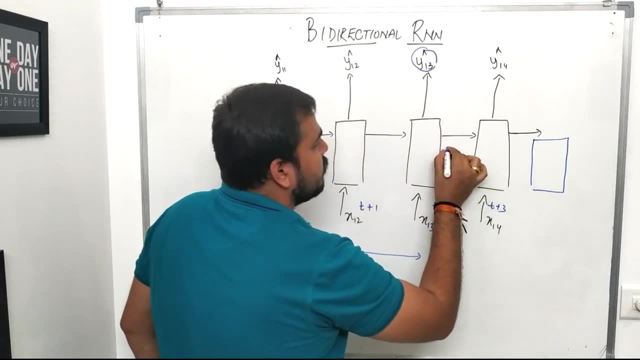 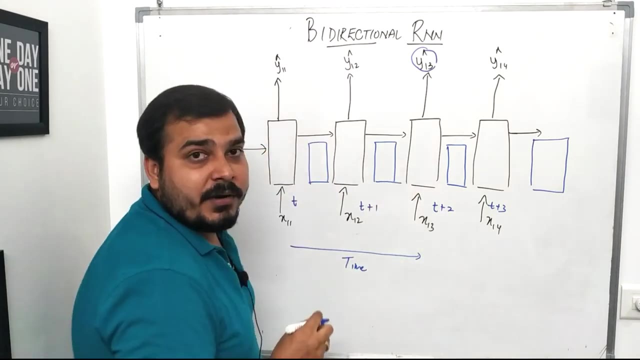 okay, so this is the same RNN. we will try to take it, okay, I'll say it, as backward layer RNN. okay, and I will just change the direction, okay, of the information. that's it. so first for that, what I can do is that I can create one RNN here, another here, another here and another here, right, so this? 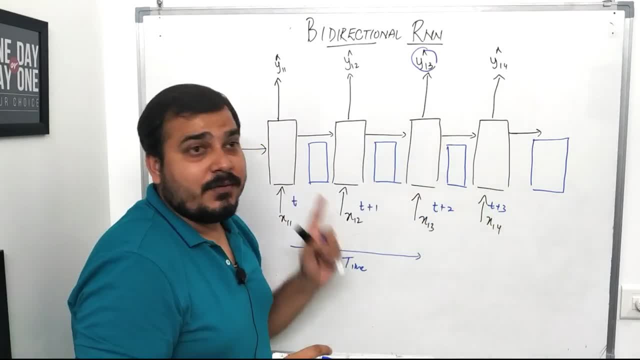 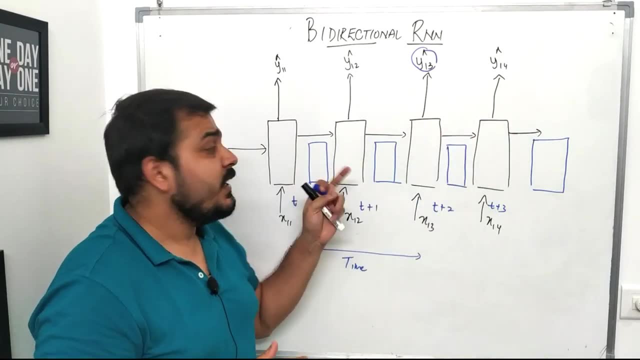 is my same number of RNN, like how we had in the forward information. remember, guys, backward propagation is different. okay, here the information passing direction I'm talking about right- in this case it is passing unidirectional right. so this is my same number of RNN, like how we had in the 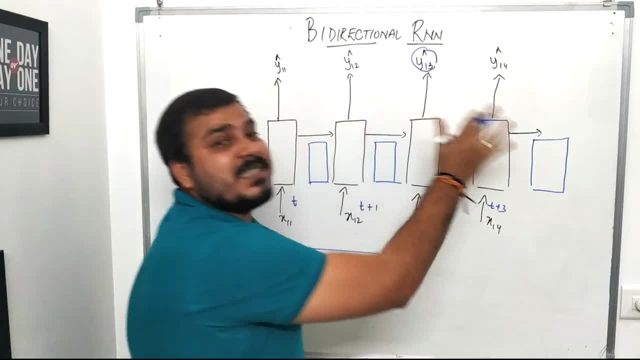 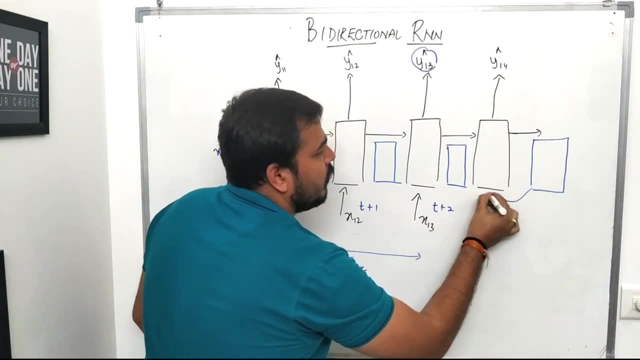 passing in one direction. what I'm going to do, I'm just going to take the same number of LSTM hidden layers. what I have taken, I'm just going to reverse the direction. now, in order to reverse the direction now, this, I'll just rub this. the information will get passed like this then from: 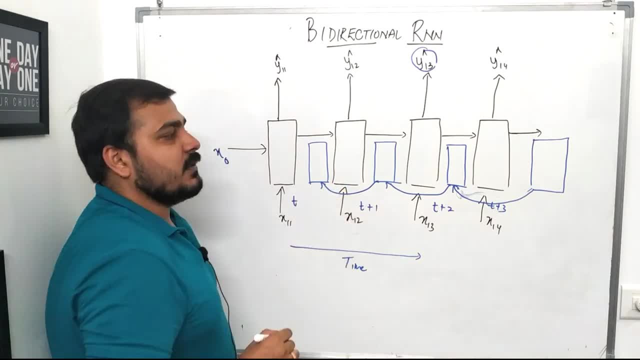 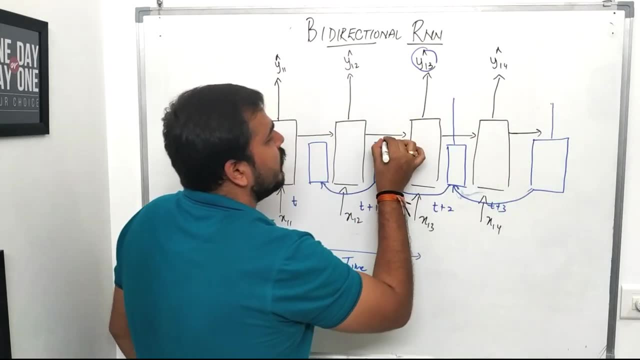 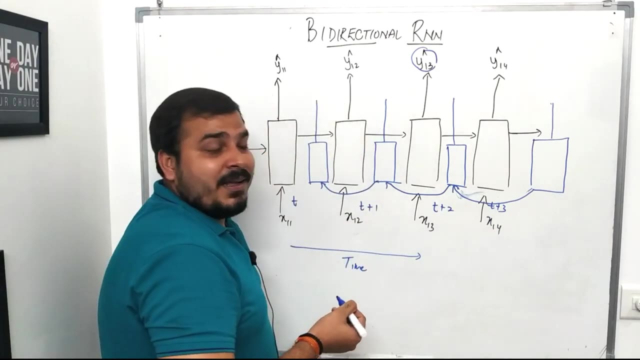 here it will get passed like this and from here it will get passed like this. right, but we also know that we get an output of from here. we also get an output from here. we also get an output from here. but the most important thing is that, where does this input goes on right? remember this. X14 will. 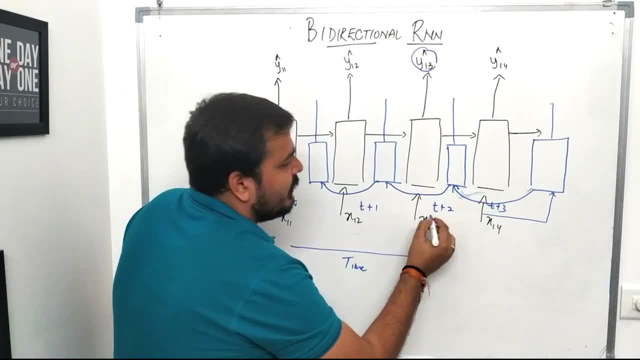 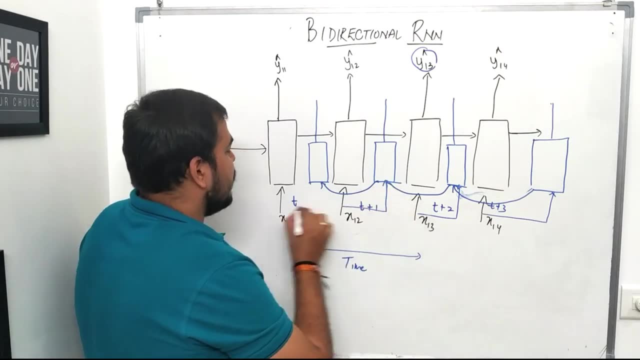 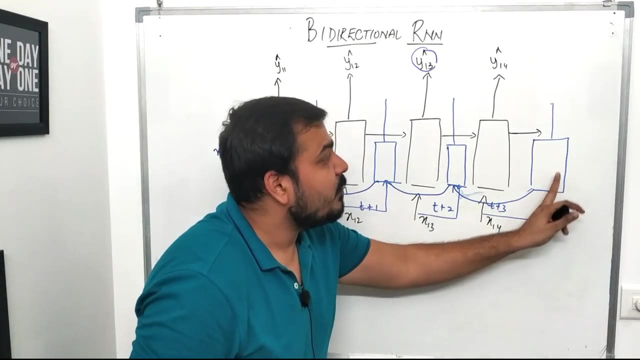 be my input to this particular hidden layer, then X13 will be the input to this layer, X12 will be the input to this and X11 will be the input to this. so understand from the reverse direction. I am giving this information to my LSTM, I am getting my output and this output will be combined. 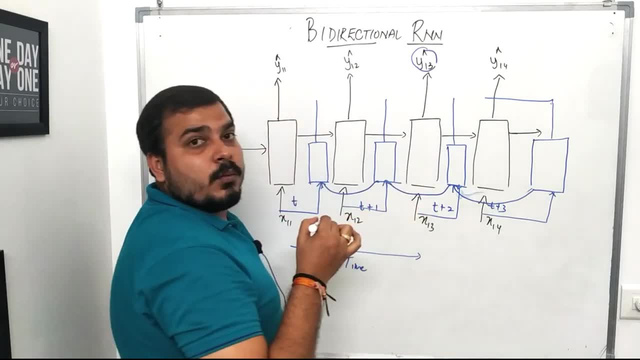 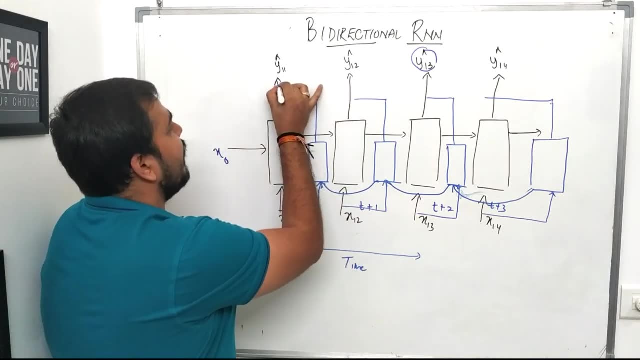 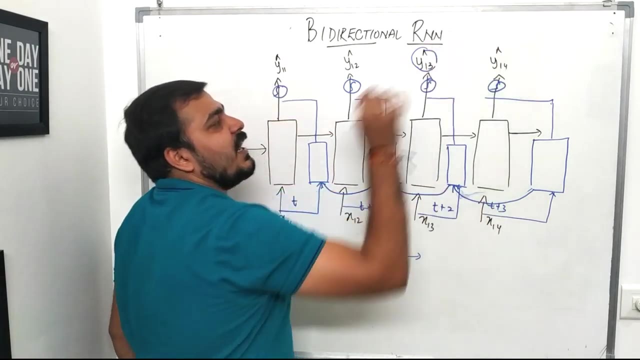 by the unidirectional app Will be combined to this one. Similarly, this will be combined. This will be combined. This will be combined. and remember, over here We have something like sigmoid function, because I'm considering this is a classification problem, So this passes through a sigmoid and finally we get the output. Now, what is happening over here? 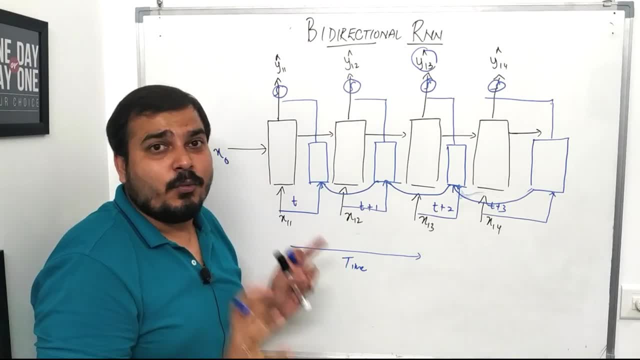 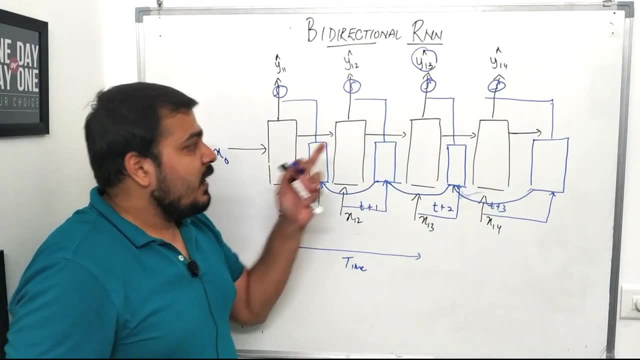 What is just happening by using this simple architecture? What we have done? We have just taken Additional layer of LSTM, We have just reversed the direction of the information. Okay Now, whenever I want to compute y1, 3, Understand, I have the information of X 1, 1, X 1, 2, X 1, 3. 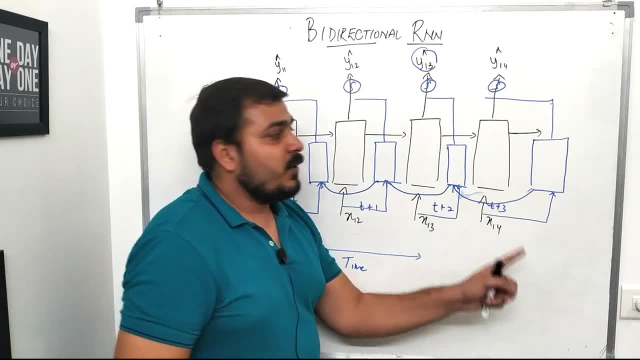 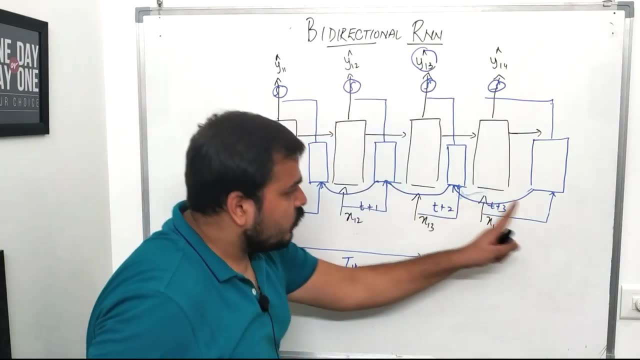 I also have the information of X 1- 4, because I understand this input is going here and this information is going here and, Based on this, this information is going here right. So, in short, I am getting the X 1- 4 information in the backward direction. 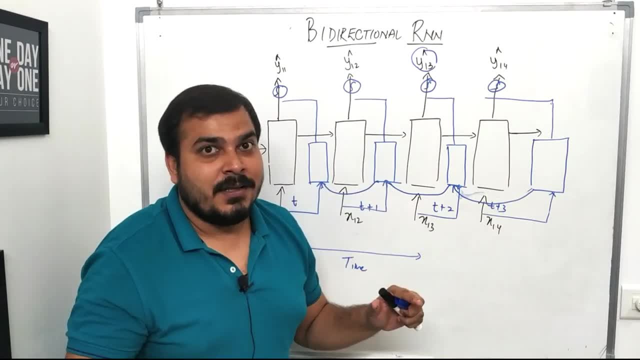 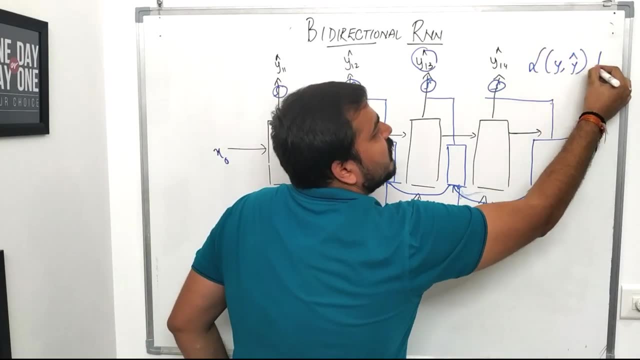 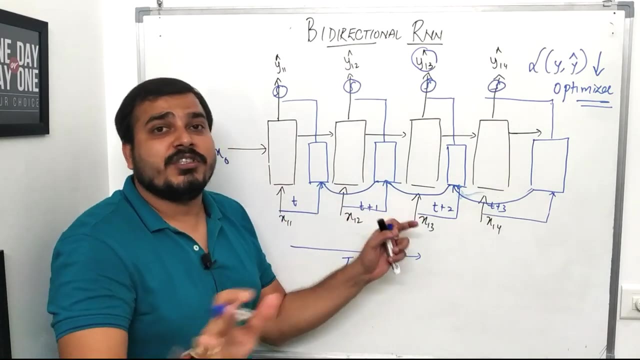 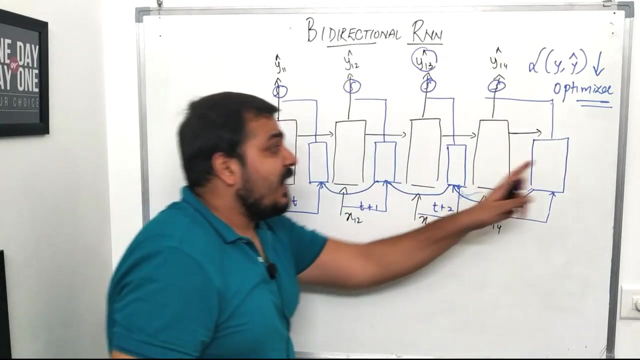 Again, understand back. propagation is different. You know, once you get your output, then with respect to that, you compute the loss, and This loss needs to be optimized by an optimizer. It has to be reduced. That step will be almost same. Only the thing that we are doing over here is that we are adding an extra LSTM layer and the information is passing through. 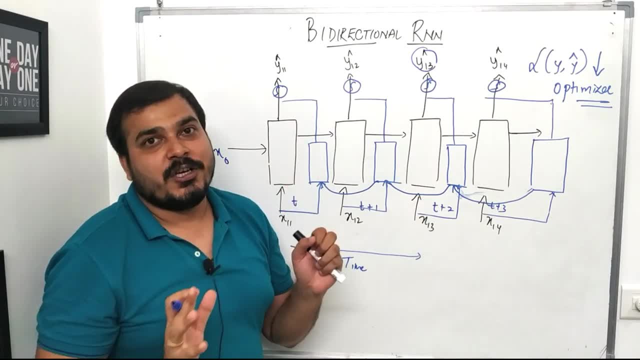 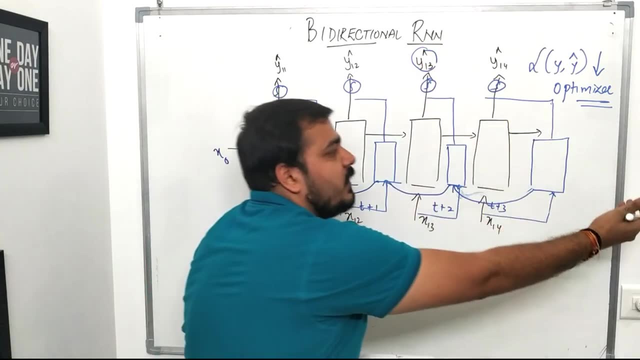 the reverse direction. right, that is what we are actually doing, and by this, this y 1, 3 is able to now get all the information of the previous word and of the Upcoming words itself, and by this it will be able to predict in a proper way. 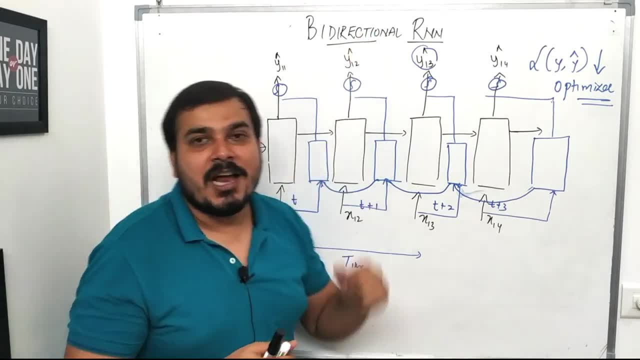 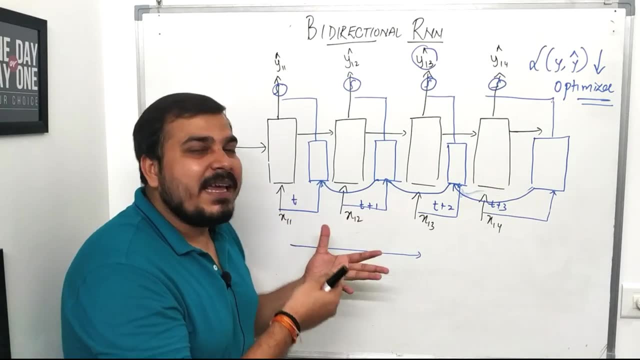 Now let us go ahead and try to understand. when should we use bi-directional RNN? So, guys, bi-directional RNN can be used for most of the NLP tasks because, understand, over there We will be getting the input right, the complete input, and by this we can also 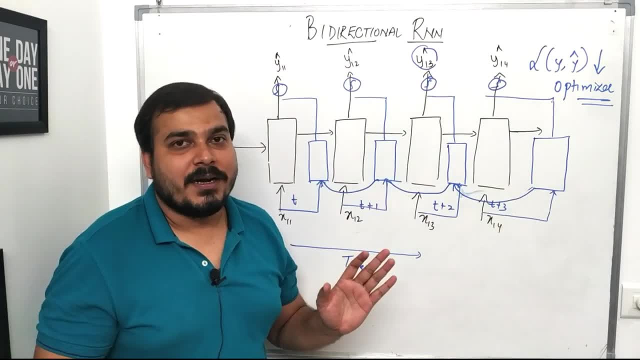 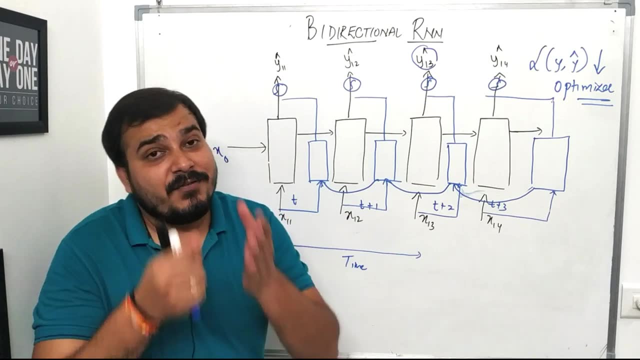 understand the future words with respect to the output that we want to predict, because the output will be predicted on the previous word also and based on the information of the future words also. so Definitely, for most of the NLP tasks, bi-directional RNN will work. 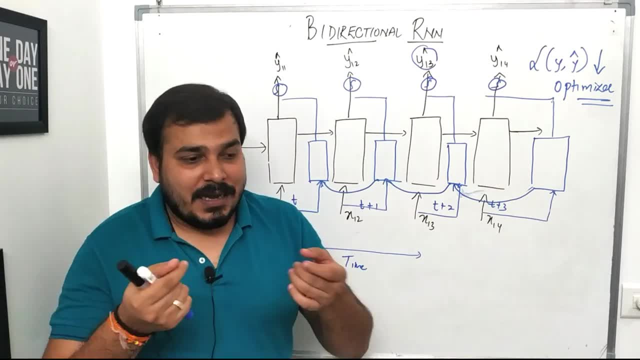 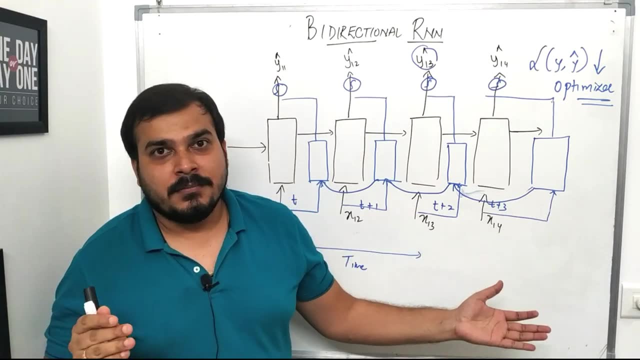 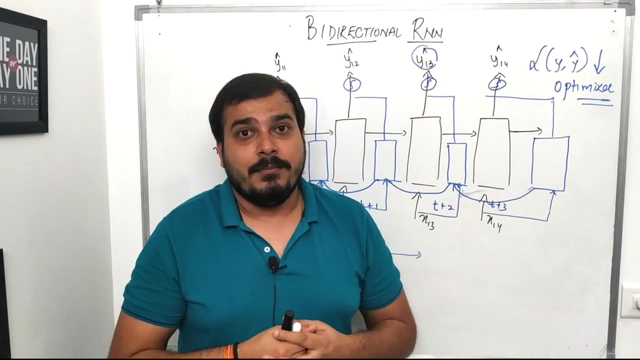 Well, right, for which scenario it may not work Well if I give you an use case: speech recognition now. in speech recognition You may not get the input all at once. you know you will be getting with respect to the time. So in this scenario your bi-directional RNN will definitely not work Well. it may give you a less accuracy. 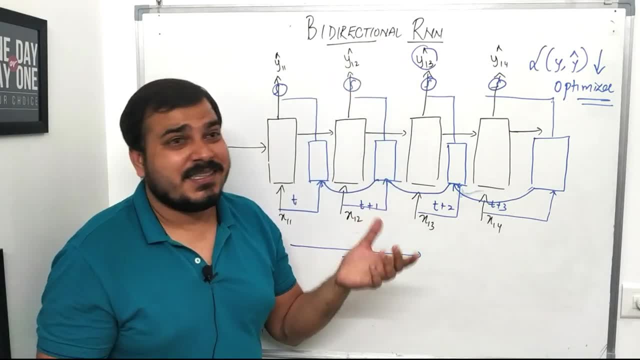 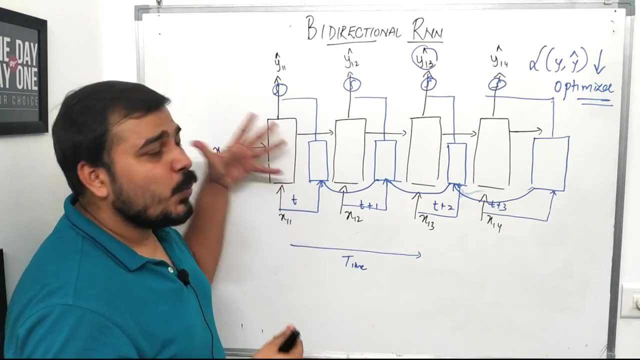 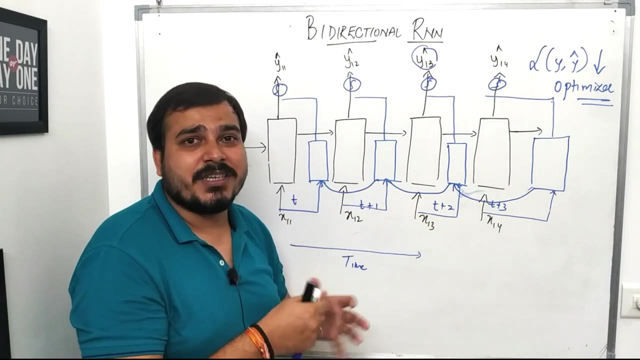 One more disadvantage of the bi-directional RNN is, guys, it is pretty much slow and compared to the normal LSTM RNN or the simple RNN, because, understand, over here We are taking the exact replica of the same layers, you know, and we are just passing the information in the bi-directional way. 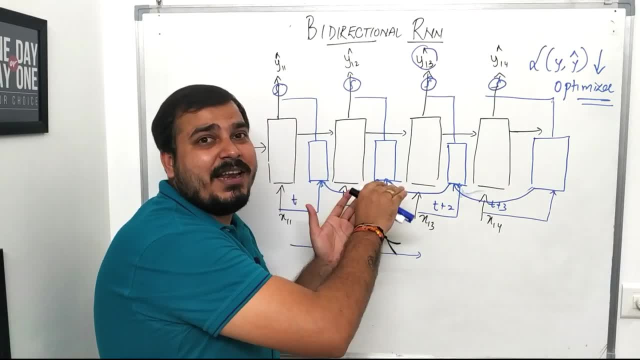 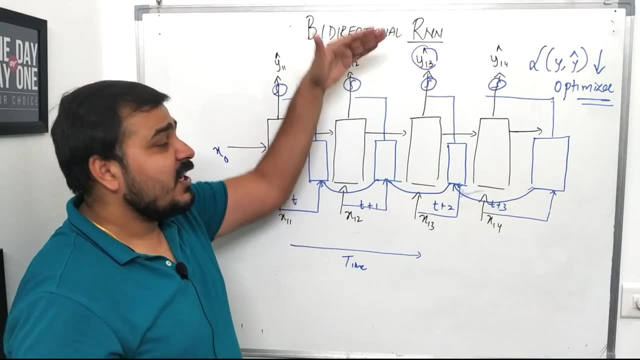 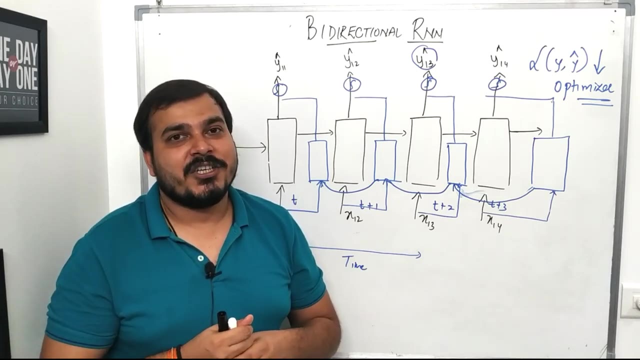 So definitely you can understand, with respect to each and every layer and when we are using cascading layers. You know, when we are using some stacking layers of LSTM RNN or bi-directional LSTM RNN, at that time This will work pretty much slow. So this is the only disadvantage with respect to bi-directional RNN.